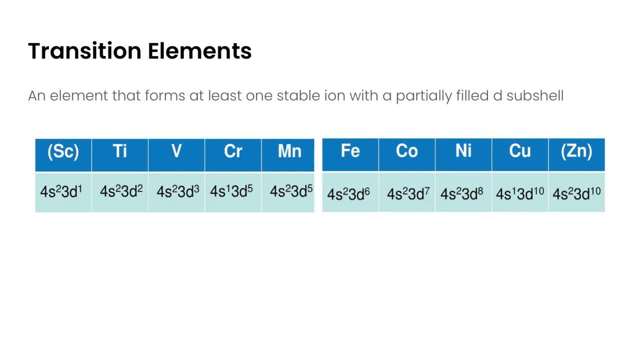 In this video we're going to take a look at the first row d block: transition elements. So the first thing we kind of want to take a look at is what is a transition element Like? what is the true definition for a transition element? Well, the definition says that it's an element that 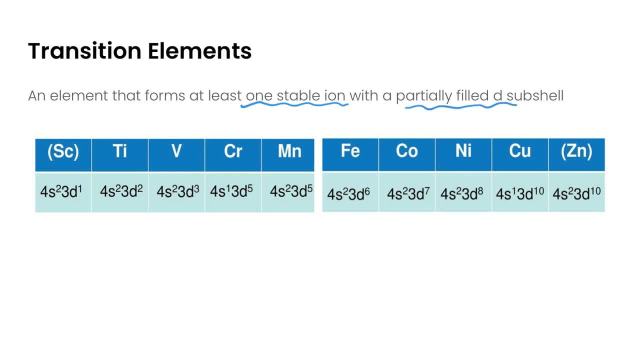 forms at least one stable ion with a partially filled d subshell. So looking at that and going across that first row d block, all of the electron configurations are shown here for the atoms themselves, not the ions. but if we were to form ions, zinc only forms a two plus ion. 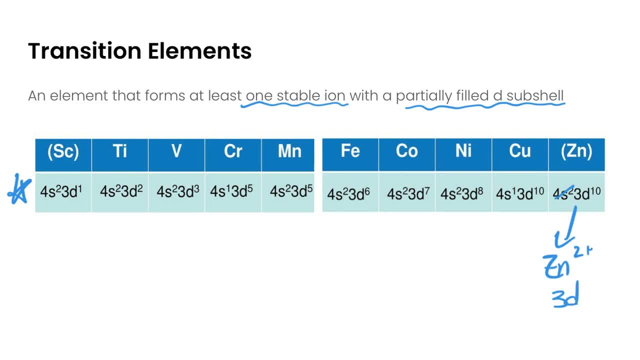 and so when it forms a two plus ion, it only has 3d 10, and so it doesn't actually fit the definition of a transition element because it has a fully filled transition element. So if we were to take a look at the first row d block, 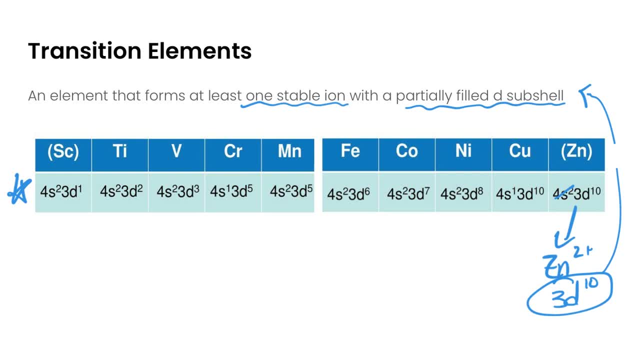 filled D subshell. There is no partially filled D subshells in a zinc two plus ion. So that's why it's in brackets here, because it's not really a true transition element. Scandium, on the other side, is also kind of questionable because for the most part it forms a plus three ion, which means 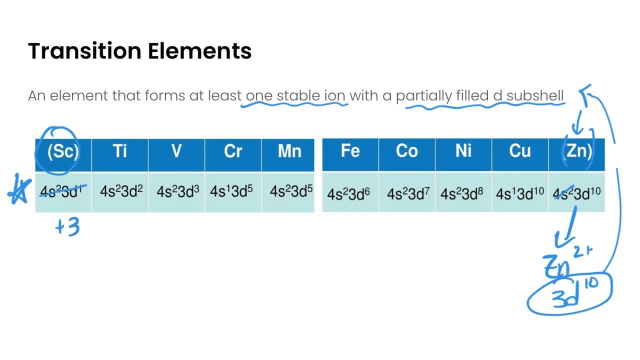 it has none of these electrons, So, again, doesn't have a partially filled D subshell. There are some compounds, though, that have a plus two charge, although even that's a bit questionable in terms of whether it's actually a plus two. For the sake of simplicity we'll include it as a transition. 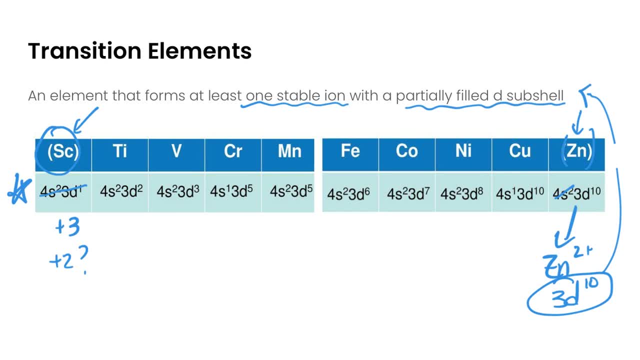 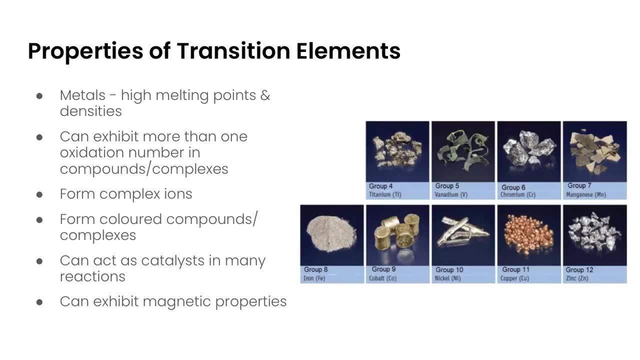 element for now, but know that there is. it's pretty questionable as to whether it is one or not. Now, transition elements have some pretty characteristic properties. So just kind of showing you some pictures of all of the different transition elements here as you go across period, the period for that first row, D block, In terms of properties, they're metals, They have. 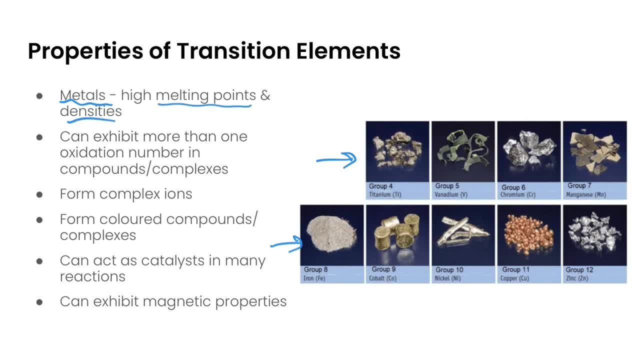 high melting points and densities. They can exhibit more than one oxidation number. in compounds and complexes They form something called complex ions, which we're going to come back to in another video and take a closer look at. They also form colored compounds or complexes. Again, I'm going to 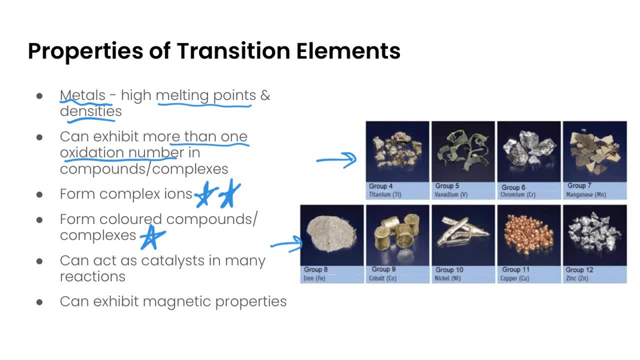 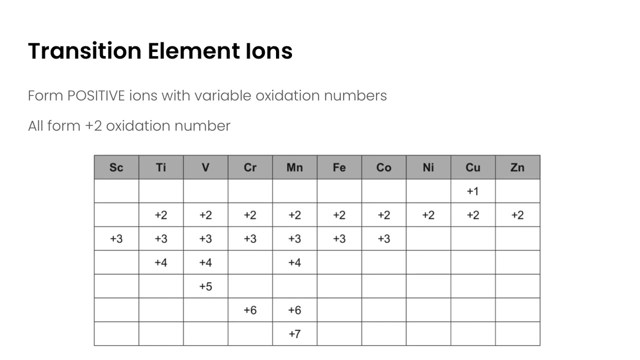 create another video that's going to go into depth about what that looks like and why they form colored complexes. They can also act as catalysts in many reactions. They are great catalysts And then they can exhibit magnetic properties. Now, one of the properties I just said is that transition elements do form positive ions with. 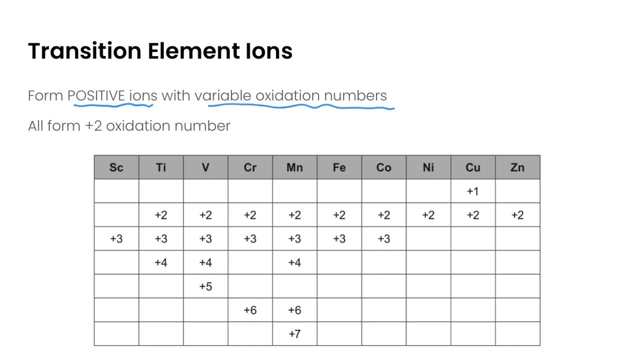 variable oxidation numbers For all of the transition elements. they all do form charges of plus two. The only one that doesn't is scandium, although that one, like we said that one, is questionable. But they all form a plus two oxidation number And that's because their electron configurations 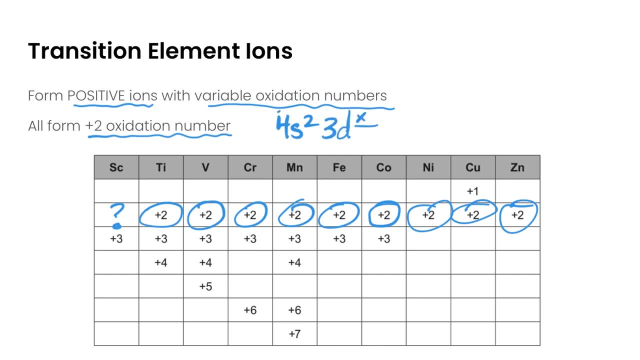 are 4s2 and then 3d some number. So those 4s2 electrons coming out gives you the plus two oxidation number. Now, when we're removing electrons from the 3d, it doesn't really follow the rules in terms of you know what's going on. So we're going to have to figure out how to. 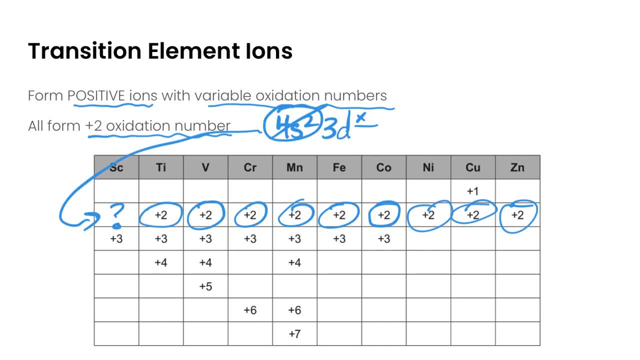 get rid of the 3d electrons in order to make a full valence shell or a noble gas configuration. They play by different rules, So that's why we get some of these variable oxidation numbers here. Okay, so you can just kind of look at the variety. quite a few form a plus three ion. 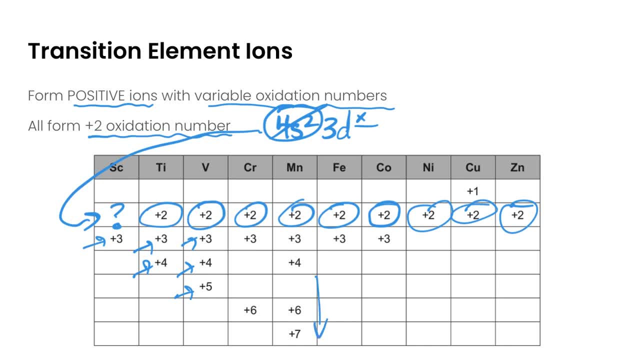 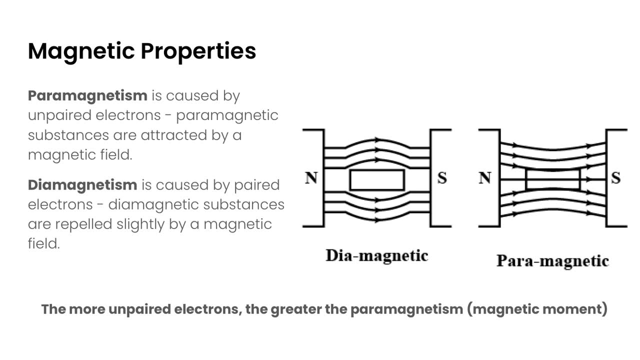 some form plus four, all the way up to manganese, which can form a plus seven oxidation. Now, one of the other properties I did mention was that they have magnetic properties. And so what do we mean by magnetic properties? Well, there's really two types. 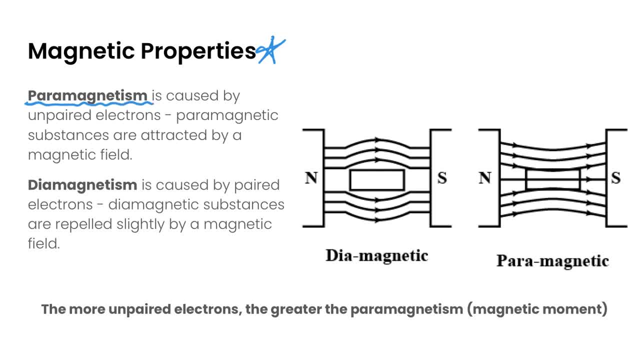 There is something called paramagnet magnetism And that's caused by unpaired electrons. So the paramagnetic substances are attracted by a magnetic field. So if we were to put a substance a magnetic field, If you're not quite sure what a magnetic field is, that's okay, It's just all. 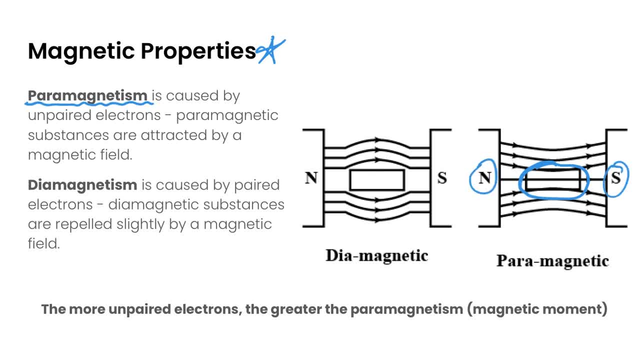 these lines here with sort of this north and south component. My physics is terrible, So you know this is about the extent of my knowledge too. But if we were to put a material in here and it was paramagnetic, then that magnetic field or those lines are attracted to that. 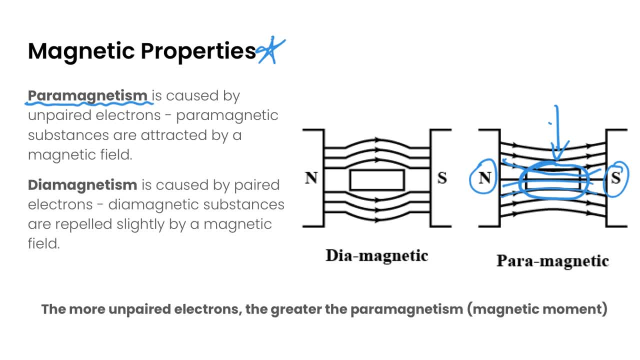 object. All right. if we have something that's diamagnetism, then that's caused by paired electrons And so diamagnetic substances. when we put that in a magnetic field they're repelled slightly by the magnetic field. So we get this, you know, skirting around these objects within 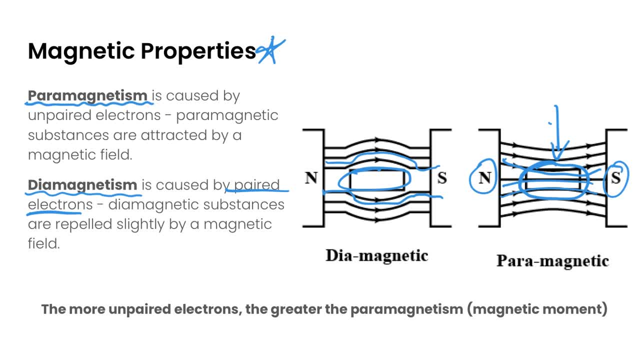 a magnetic field, So kind of. the key thing here is to look at whether you have a substance that has unpaired electrons or paired electrons, And specifically we're going to be looking in the d orbitals And we're going to be looking at whether they are paired or unpaired The more 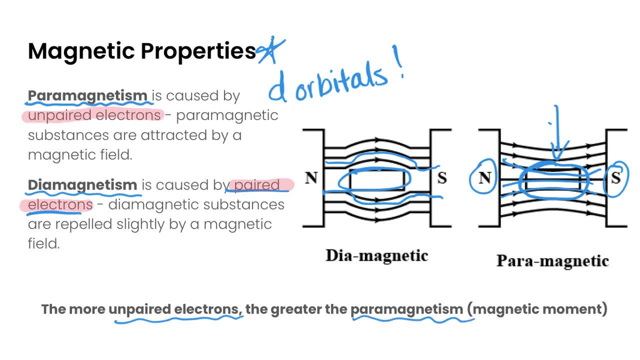 unpaired electrons you have, the greater the paramagnet magnetism is. So that's just kind of another property that we need to know. Okay, so this is all great and dandy, We've got some definitions here, But what does this all mean? 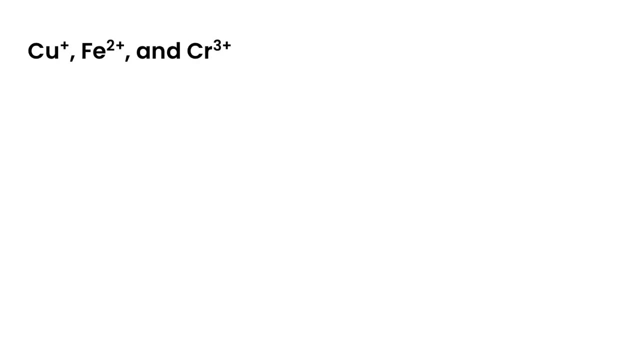 What does it look like for some of our transition metals? So let's take a look at a few. Let's start with a copper two, or sorry, a copper one plus ion that has an electron configuration of. we'll just do the shorthand, argon and 3d 10.. So this one here, 3d 10,, means that we're going to have 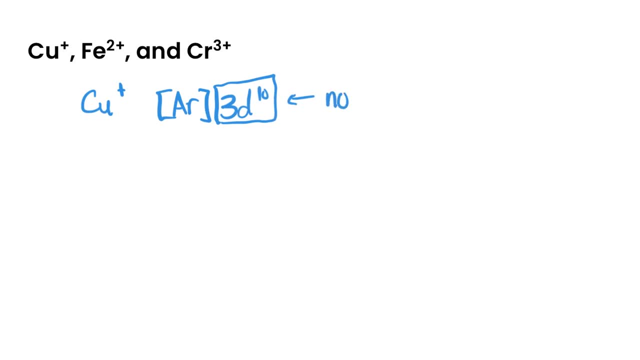 no unpaired. So there are no unpaired electrons in those 3d orbitals. That means that it is dia, magnetic, magnetic. there we go, I can spell it Okay. so if we were to put that in a magnetic field it would repel the magnetic field. Let's look at another one: Fe two plus now. Fe two plus. 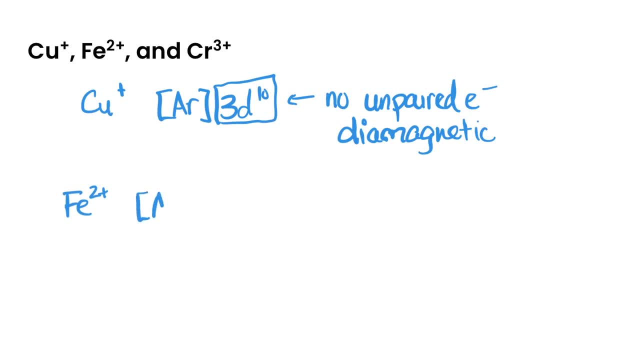 has a argon, And then it's 3d six. So if we look at those 5d orbitals, then we're going to put one in each And we'll double up on one. So in this case we have- let's just kind of highlight them- 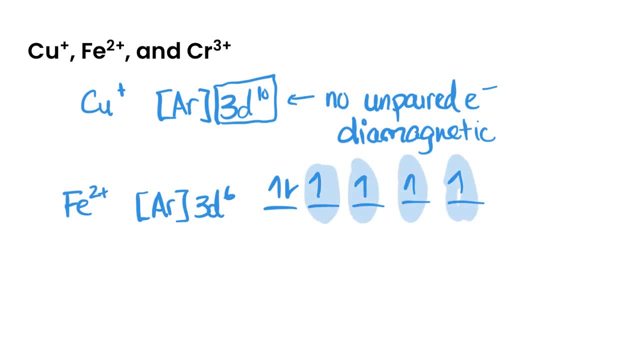 here we've got one, two, three, four unpaired electrons, So four unpaired electrons. If we have any unpaired electrons, it means that it is paramagnetic, So paramagnetic, okay. Now looking at something similar. so let's look at chromium three plus. 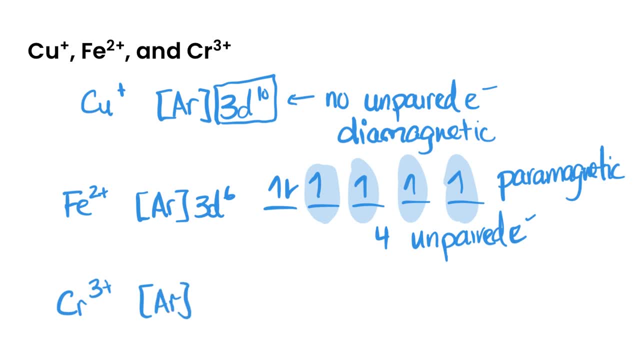 that has an electron configuration of argon and then 3d three. So again, if we take our 5d orbitals, 3d three means that we have one unpaired electron and three orbitals here. So we've got one, two and three unpaired electrons. Again, it is paramagnetic. 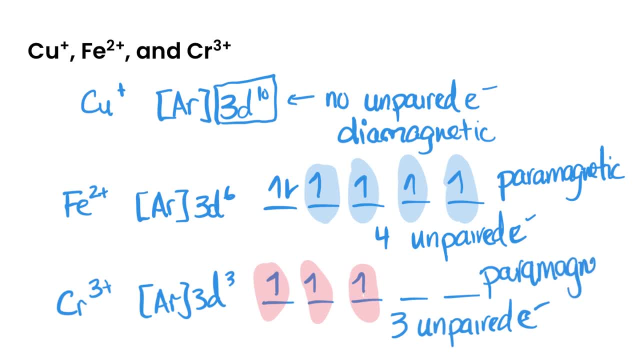 So it's paramagnetic, which means it would attract a magnetic field. but we would say that it is less paramagnetic than the Fe2 plus ion, because there are only three unpaired electrons here versus four. so there's more paramagnetic or paramagnetism in the Fe2 plus versus in the chromium 3 plus ion.